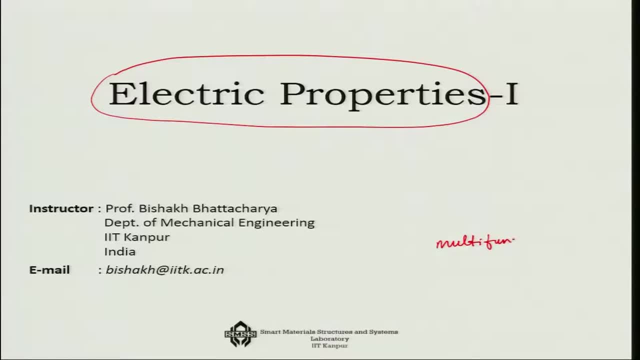 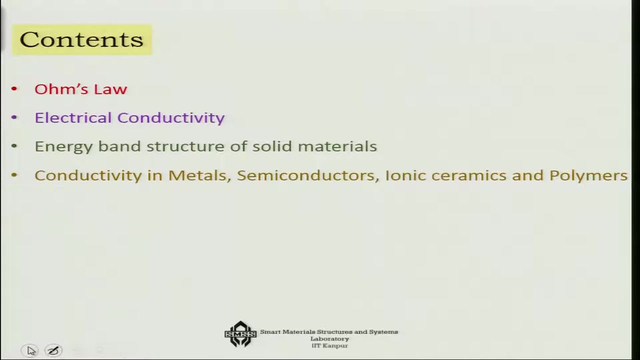 today- okay, In fact very shortly- they are also called functional materials. So functional materials actually solve more than one purpose. They not only solve the mechanical purpose, but they also solve some electrical or maybe thermal or maybe optical or maybe magnetic, you know- functions they actually take care. So in this particular talk we are going 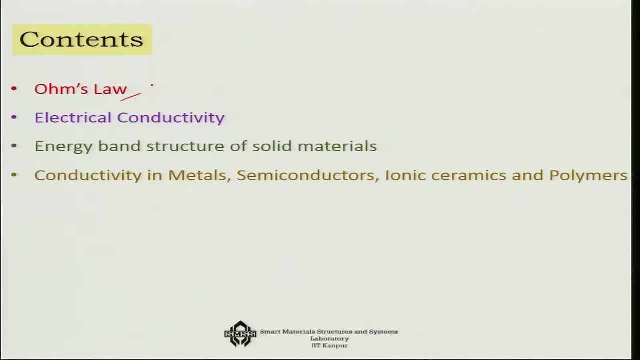 to talk about the Ohm's law, which you all know, but for the sake of you know completeness, we should discuss it. Electrical conductivity, energy band structure of solid materials, and then conductivity in metals, semiconductors, ionic ceramics, particularly that group of ceramics which has the ionic 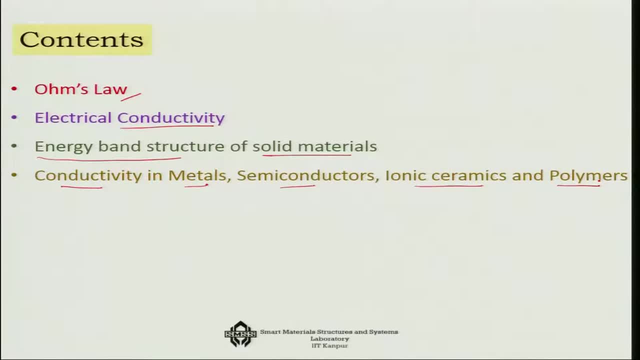 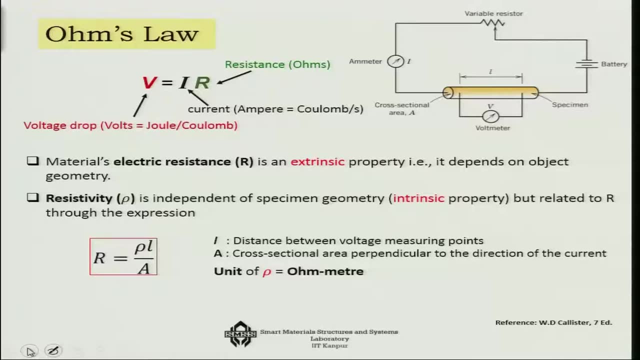 bonds and the polymers. So this is what we are going to talk about in today's lecture. So let us first start our life with the Ohm's law. So let us start this from your school days- that the voltage drop in a you know circuit. 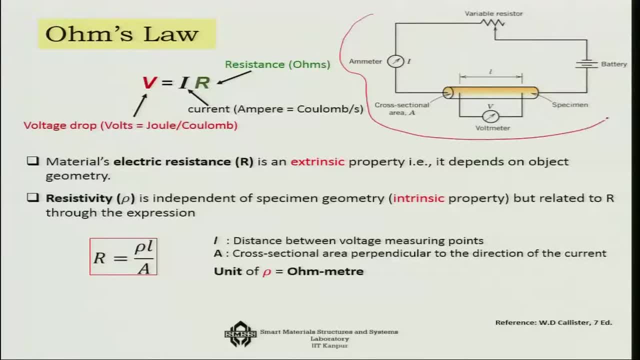 let us say: this is what is our circuit here. okay, And we have a battery, which is the power source, and then we have a resistor. It can be a variable resistance, which means you can change the resistance of the resistor. We have a ammeter which can actually measure. 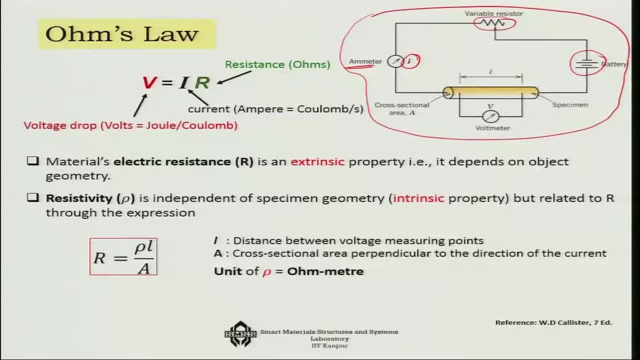 the current and then a part of. So this is the current that is flowing in the ohm's law, This is the current that is flowing in the loop, okay, and you have to complete the loop. Now there is one part here where you are actually putting a new material. let us say whose resistance. 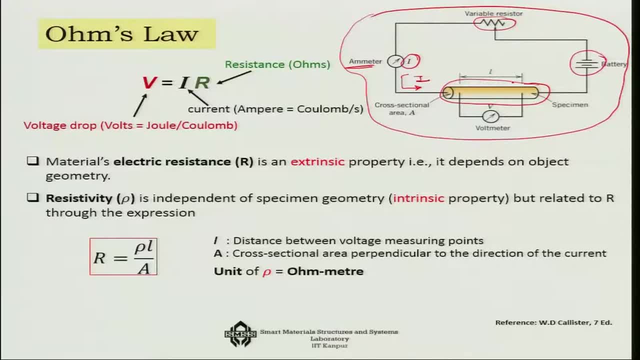 is what you are interested to find out. So you know what is the cross sectional area of the material and you know what is the length of the material and, as you know the current I, I have to find out what is the voltage across it. okay, through a voltmeter, assuming that. 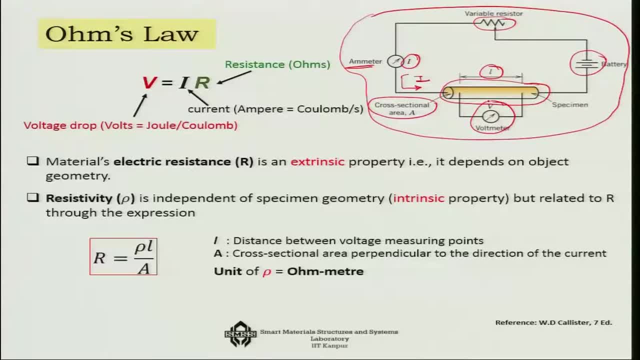 the voltmeter is going to take minimum amount of resistance So that it is going to actually measure the voltage drop between the two without you know adding to the voltage drop, and then the circuit is complete once it is coming back to the battery. 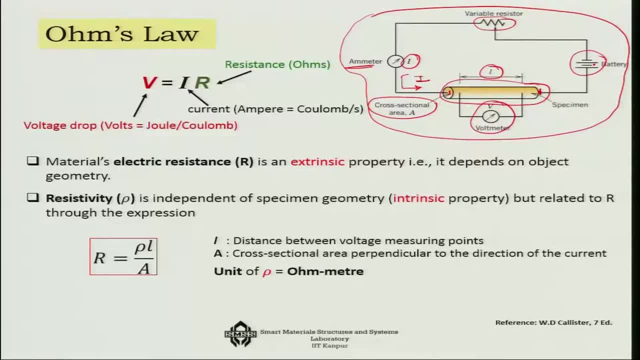 So, with this kind of a simple circuit system, if you actually you know, note down that what is the voltage drop Okay, and what is the current from the ammeter, then you will be able to find out that what is the resistance of that particular length, of the particular material. Now, this resistance. 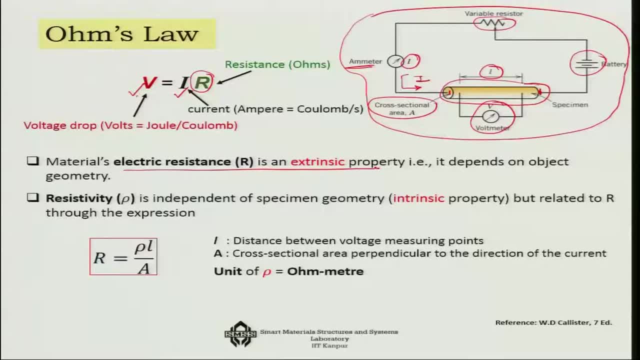 is an extrinsic property because it not only depends on the material property, but also on the cross sectional area, on the length, etcetera. Okay, So the intrinsic material property that you should go for is called resistivity, which is also denoted by rho. So rho for density, roe for resistivity. we should not actually 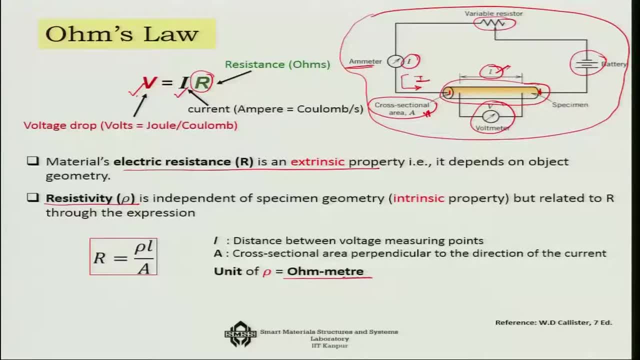 confuse between the two, because the unit here is ohmmeter. okay, Now with respect to the extrinsic property, resistance, the relationship is simply given here as: R equals to rho times L over A. a. that is the relationship. So once I know this material property of resistivity, once, 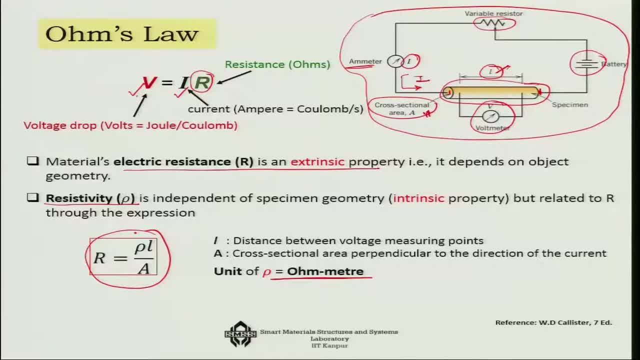 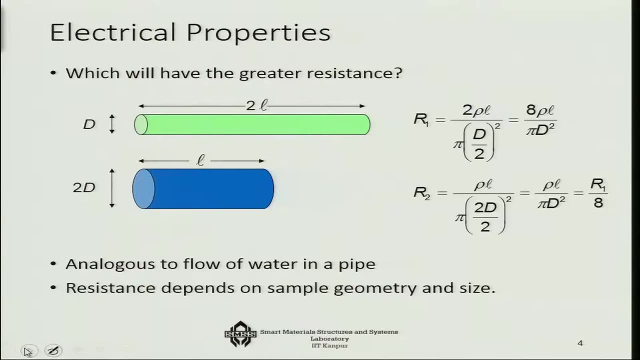 I know the length of the material in the wire form and the cross sectional area, I can find out what is the actual resistance it will be, or the you know it will be offering when you pass a current across it. Now then, suppose you know, I take two wires, one of diameter d and length 2 L, and in the 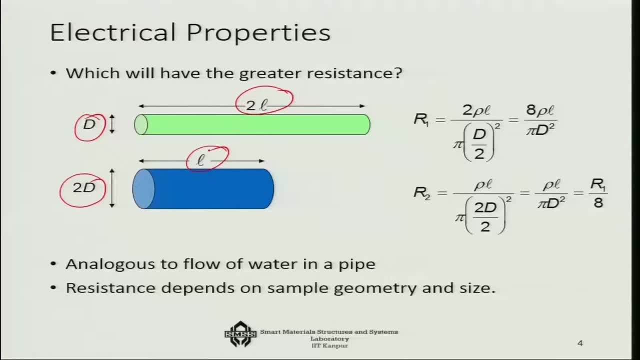 other case it is of diameter 2 d and length L. So what is the extrinsic resistance in the first case? Well, in the first case the length is 2 L and the resistivity is same rho, and the wire cross sectional area is pi d square by 4.. So it will become 8 rho L. 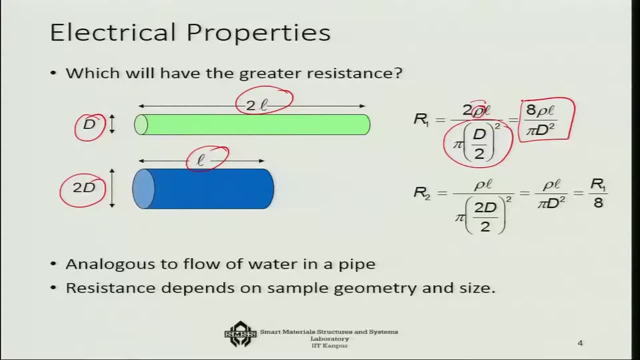 over pi d square by 4.. On the other hand, if you consider the resistance of this one, R2, then resistivity is same again. rho length is now L and diameter is double, now 2 d, So that you substitute and you will. 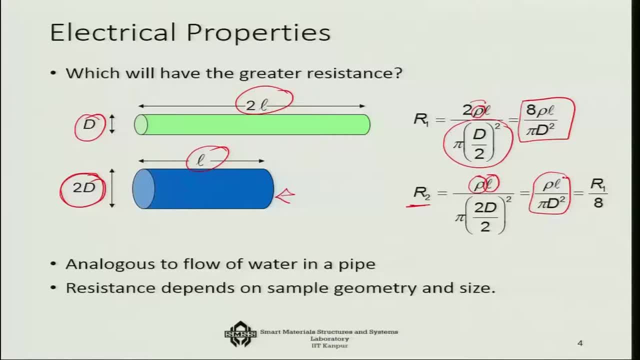 get it as rho L over pi d square. So what it means is that R2 is actually one-eighth of R1.. So what it means, It means that if I double the diameter, my resistance comes down by one-eighth. On the. 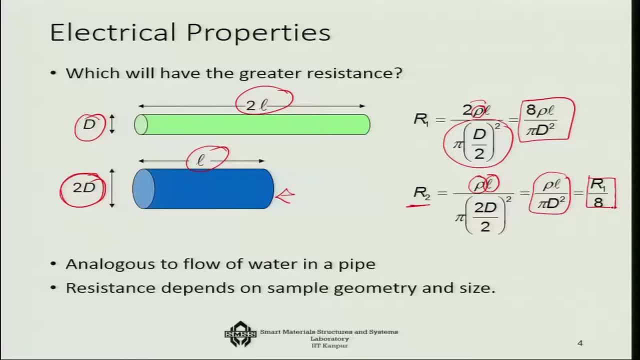 other hand, if I go for doubling the length, then my resistance increases. This is actually analogous to flow of water in a pipe, And this also demonstrates that the resistance depends on sample geometry and size, But resistivity is an intrinsic material property. 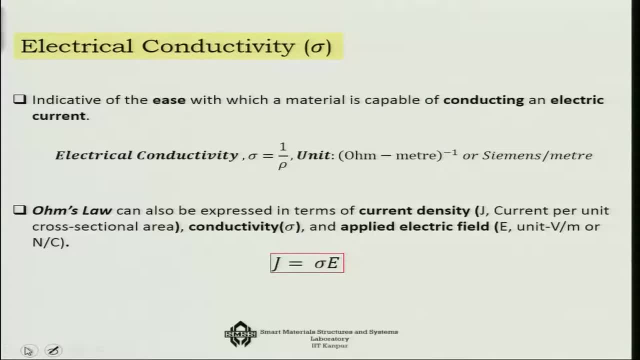 Now, similar to the resistivity, there is another very important term that we use that is called conductivity, which is inverse of the resistivity. So electrical conductivity is sigma equals to 1 over rho and hence its unit is ohm meter inverse, or sometimes people 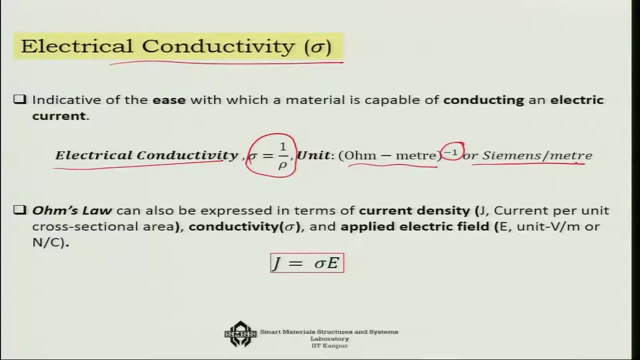 also call it as cementing. So this is indicative of the case where a material is highly conductive, and what is its level of conductivity corresponding to electric current? we can measure it with respect to sigma. Now that we know that this sigma is there with us, we can actually get a better form. 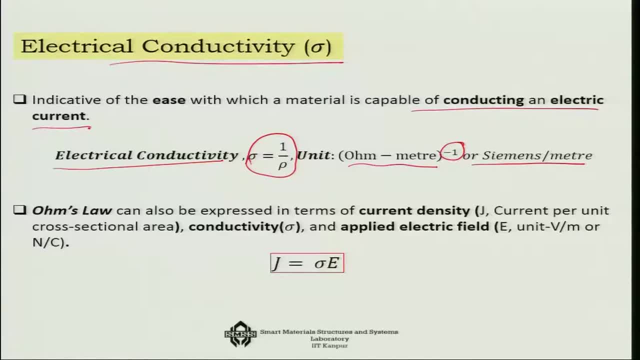 of the ohms law, now current density, J, which is current per unit cross sectional area. J equals to I, current per unit cross sectional area, and voltage. you already know that voltage equals to IR, So which means that I can write: I equals to V over R. 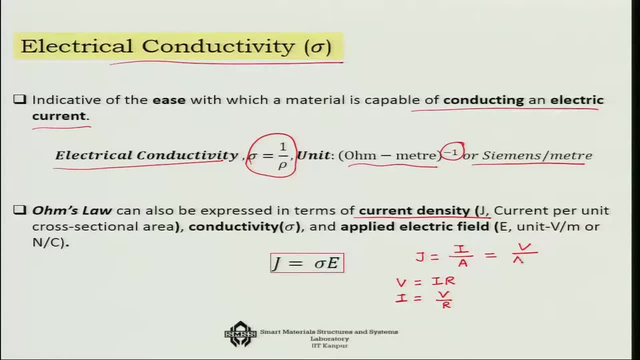 So I can write this as V over AR, right. Also, I can write R in terms of resistivity, which is rho and times L divided by cross sectional area A. So if I substitute this expression here, I am going to get it as V over A times rho, L over A. I can cross area and area. 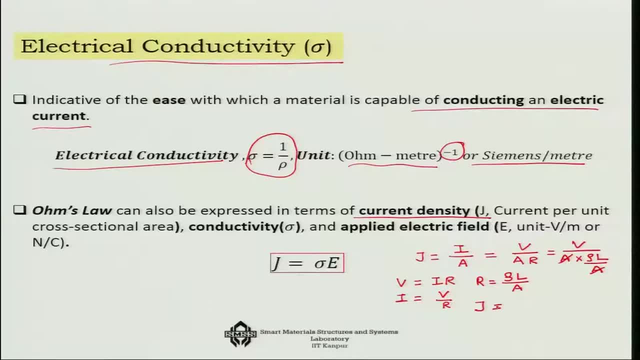 So as a result, I am getting J equals to V over rho L. And also I have already said, by definition, sigma equals to sigma equals to 1 over rho. I already said So we can write that as sigma. and this voltage per unit length is a new term. 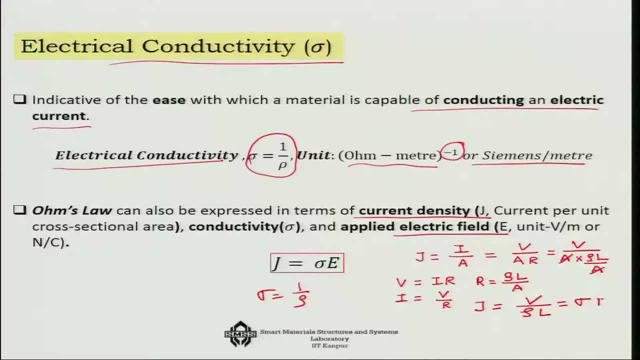 We can call it as the applied electric field E. So I can write it as: J equals to sigma E, okay, where E equals to voltage over the length. So thus we can actually get this beautiful relationship where the J- you know the current density- can be related to the applied electric field. 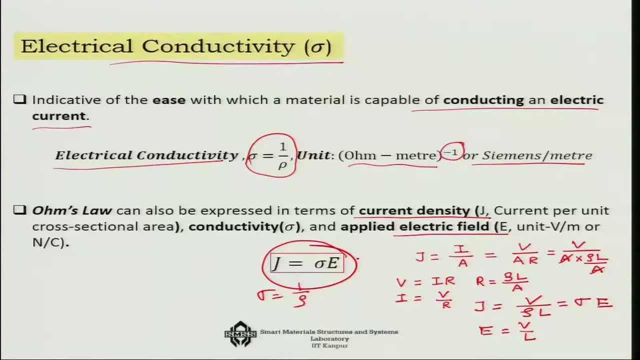 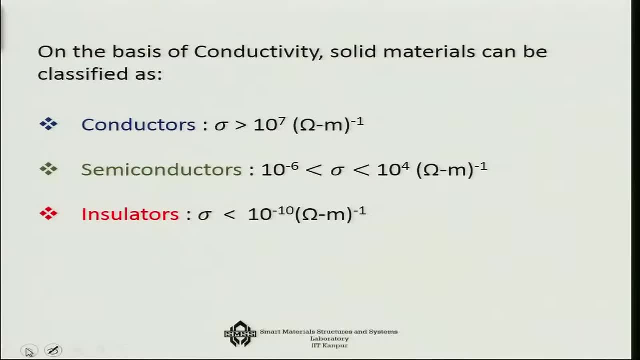 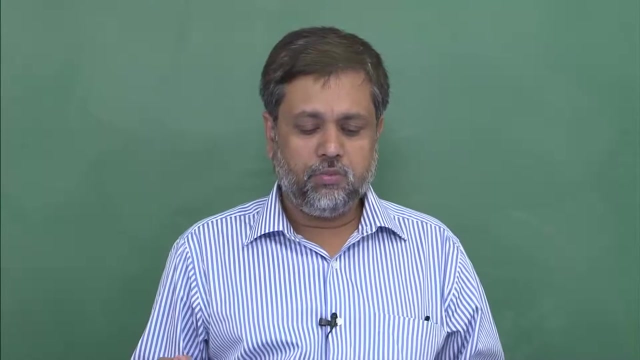 Okay, So this is the applied electric field, with the help of electrical conductivity, and that is a new form of the Ohm's law. Now, on the basis of this conductivity, solid materials can be classified into three parts: Conductors, where the conductivity is greater than 10, to the power, 7, you know, per ohm meter. 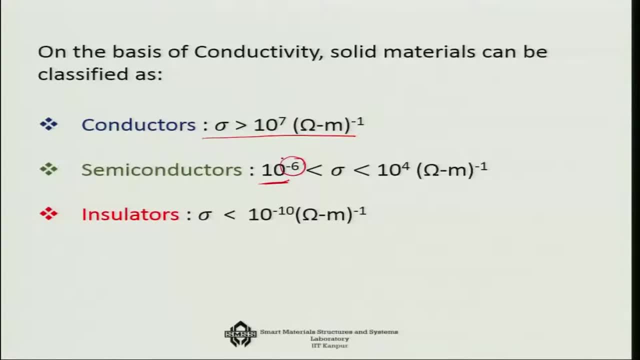 Semiconductors where it is in between 10 to the power minus 6 and 10 to the power 5.. So this is the applied electric field. Okay, So this is the applied electric field. So this is the applied electric field. 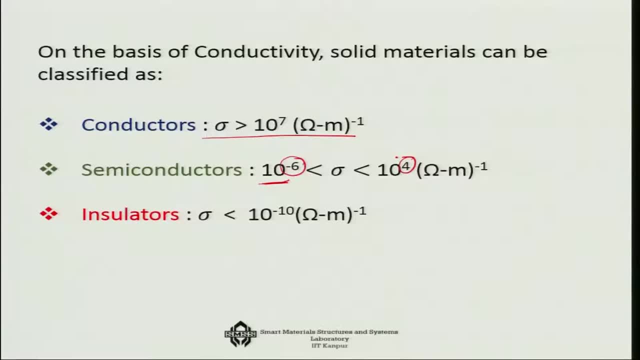 Semiconductors, where the conductivity is greater than 10 to the power 4 ohm meter per ohm meter, and insulators, where it is actually less than 10, raise to the power minus 10 per ohm meter. So let us look into each one of this now. 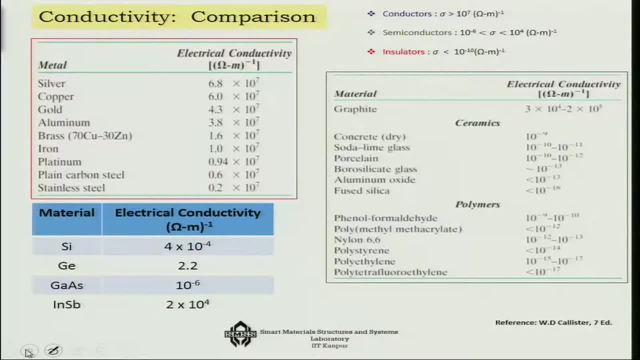 Suppose, if I look into the conductivity of the metals, where are they? Well, one of the highest conductivity is silver, which is 6.8 into 10 to the power 7 and, interestingly, all the almost all the you know, generally the material metals that we use, all of them. 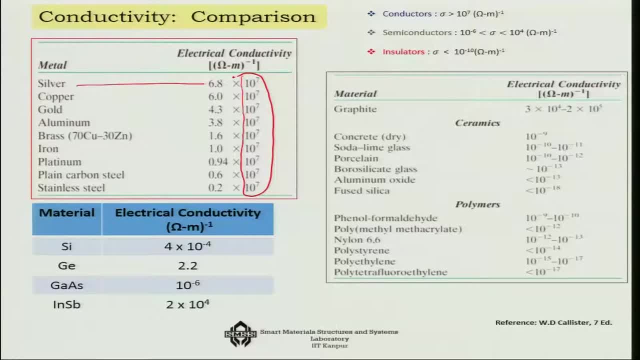 have 10 to the power 7 range of conductivity. But next to silver is copper which is 6.0, gold 4.3 into 10 to the power 7, every case. aluminium 3.8, brass 1.6, iron 1.0, platinum 0.94, plain carbon steel further lower than. 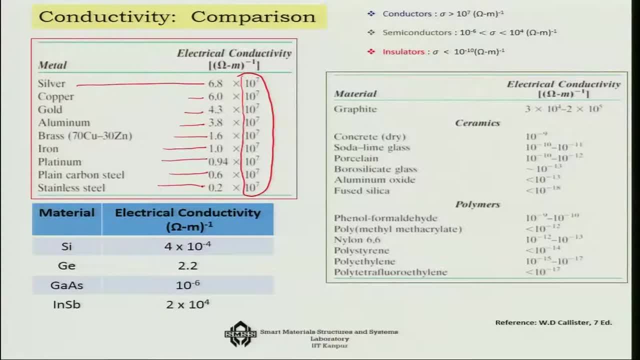 iron, because of the alloying: 0.6.. Okay, Okay, Stainless steel, because of the addition of the carbon, it is even lower: 0.2.. So that is the level of electrical conductivity. Now, if you consider some of the materials which are, like you know, semi-conductive materials, 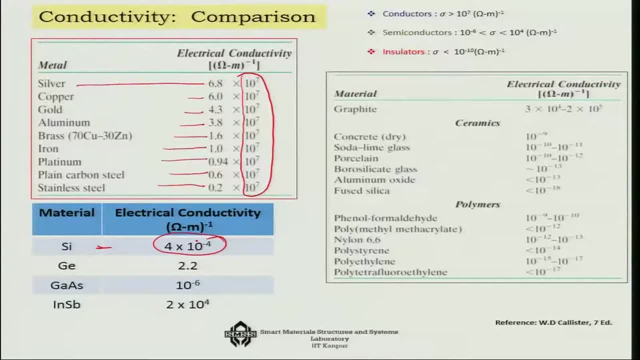 silicon, 4 into 10 to the power minus 4, germanium, 2.2, gallium, arsenide, 10 to the power minus 6, and INSB. So it is a medium based. you know this thing. alloy 2 into 10 to the power 4.. 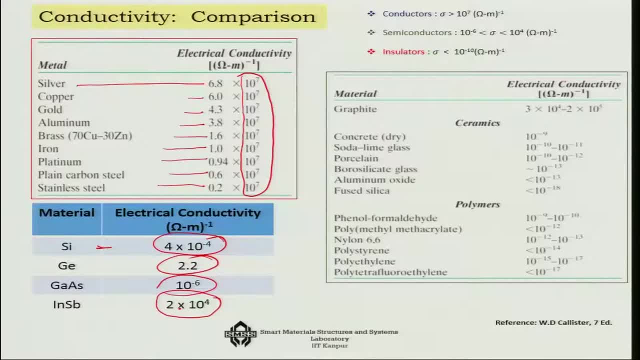 So we can see here that really the semiconductors are between 10 raise to the power minus 6 to 10 raise to the power, 4 and per ohm meter, and conductors are greater than 10 to the power, 7 per ohm meter. 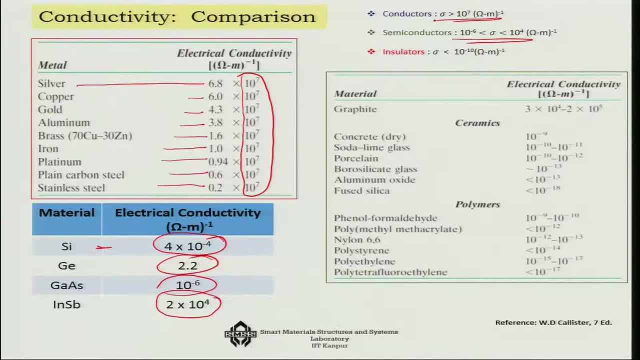 And if we consider the insulators in this list, then graphite, 3 into 10 to the power 4 to 2 into 10 to the power 5.. Then concrete, it is 10 to the power minus 9.. So you see, so low, except graphite, everything else graphite is only having a good conductivity. 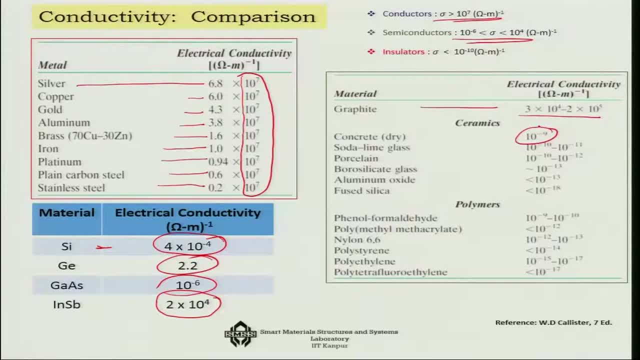 not as good as the metals, but still quite a good conductivity. Soda, lime grass: 10 to the power- minus 10 to 10 to the power minus 11, porcelain: minus 10 to minus 12.. Borosilicate: 10 to the power- minus 13,. aluminum oxide: 10 to the power- minus 13,. fused silica: 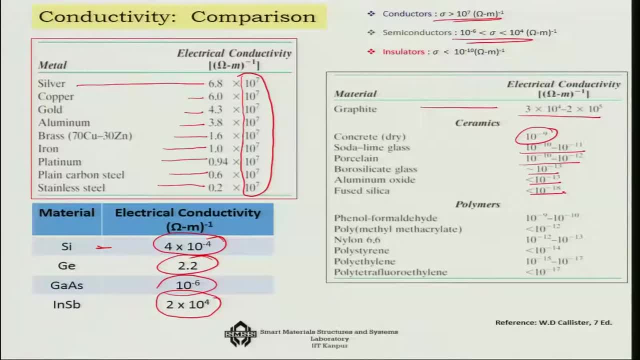 10 to the power: minus 18.. And if you consider the polymers, where are we like? phenol formaldehyde: 10 to the power minus 9 to 10 to the power, minus 10.. PMMA: 10 to the power minus 12,. nylon: minus 12 to minus 13,. polystyrene: minus 14,. polyethylene: 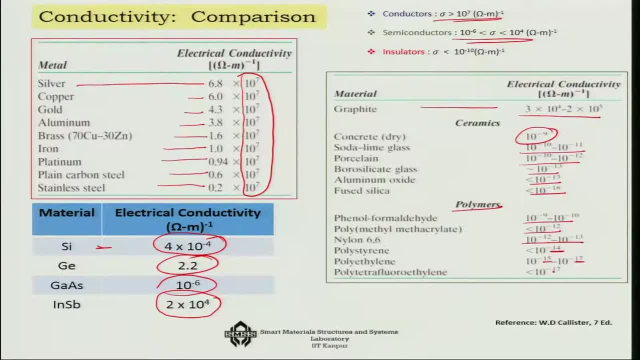 minus 15 to minus 12.. And polytetrafluoroethylene minus 17.. Having said that, again, there are some polymers like polypyrroles, etcetera, which shows much higher degree of conductivity, But we will come to it when we will discuss about the polymers. 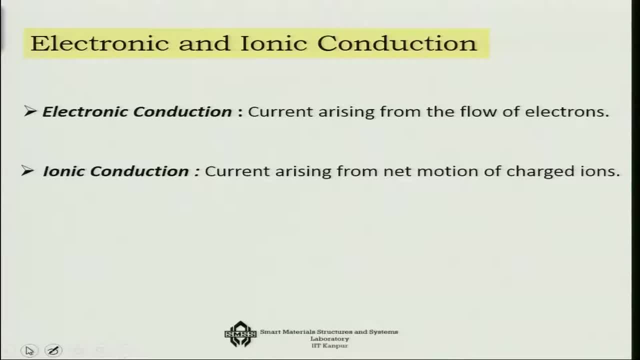 Now the next point is electronic and the ionic conduction. How basically the conduction takes place. there are two ways. One is that conduction Due to the flow of electrons, and another is the ionic conduction, where current is arising from net motion of the charged ions. 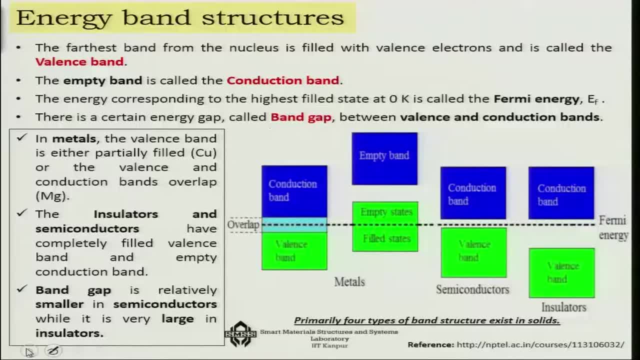 So, in order to explain that, we have to know little bit about the energy band structures. Now, the farthest band from the nucleus is filled with the valence electrons, and that is known as the valence band. So So this is, where is our valence band? 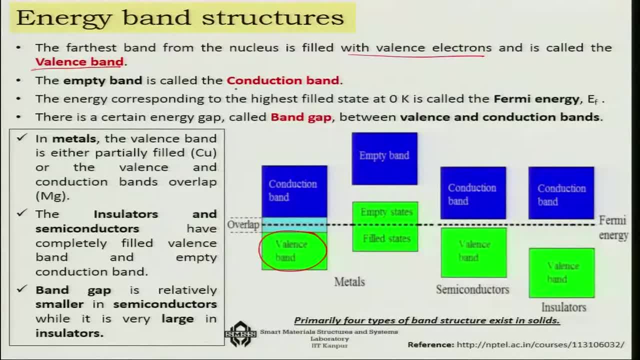 Then there is an empty band which is called the conduction band. So this is where is our conduction band. The energy corresponding to the highest filled state at 0 degree Kelvin is called the Fermi energy level. So this is what is our Fermi energy level. 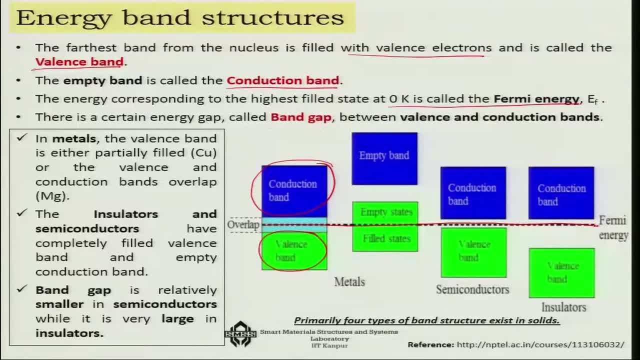 That is the highest energy state. Okay, Just keep in mind that your valence band is below this level. So this is where is our conduction band. This is the highest level And your conduction band is above this level. There is a certain energy gap between the conduction band and the valence gap, and that 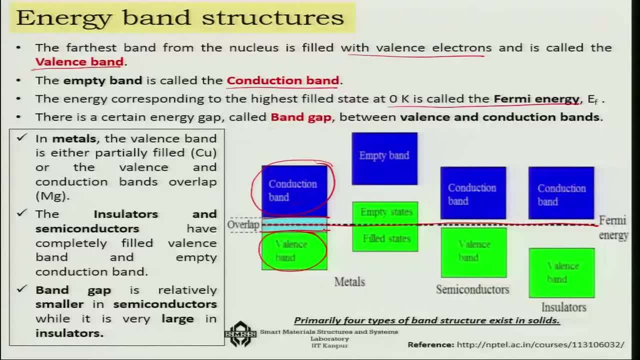 is known as the band gap. as you can see the band gap here Now, in metals the valence band is either partially filled, like copper, or the valence and conduction bands. they overlap, like in case of magnesium. So there will be either overlapping or they will be overlapping. 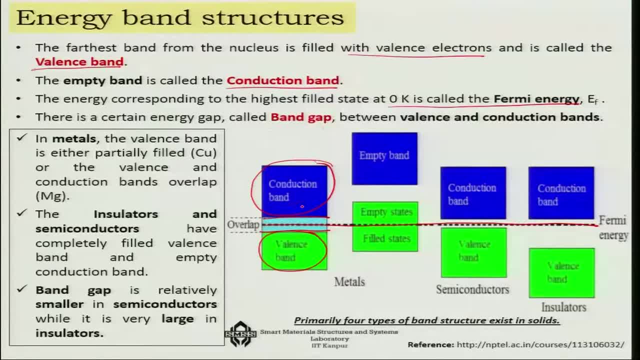 lapping or they will be partially filled. On the other hand, the insulators and semiconductors have completely filled valency bands and empty conductive bands like this: that valency band completely filled and this is completely empty. This part is completely empty, and the same thing is true for the insulators that this 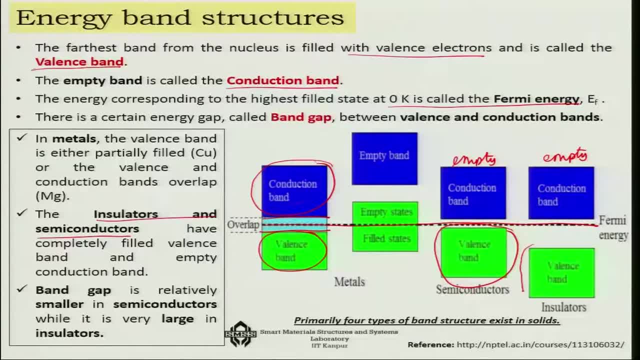 is empty and the only difference between semiconductor and the insulator is that this gap is even more, you know, in the case of the insulators. So the band gap is relatively smaller in semiconductors, while it is very large in the insulators. 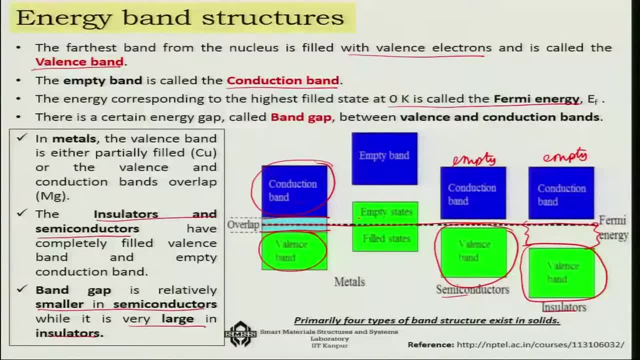 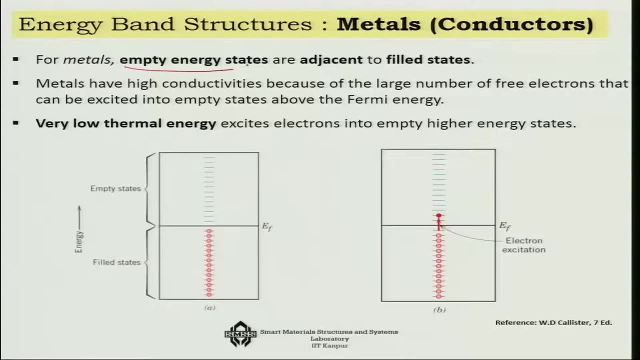 So you need to supply, in case of metals, only a little amount of energy so that the conduction band, can you know? Then start to flow the electrons and cause the generation of the current field. So for metals, empty energy states are adjacent to actual field states. they are very close. 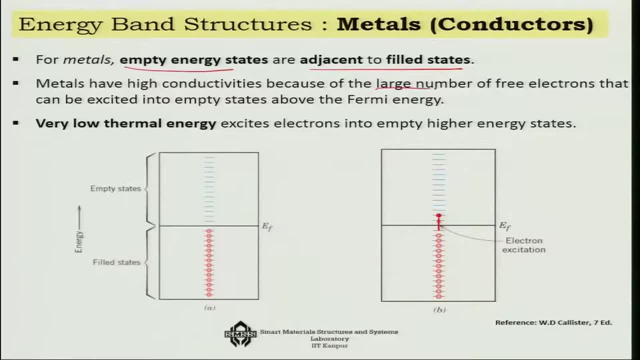 And metals have high conductivities because of the large number of free electrons that can be easily excited into empty states above the Fermi energy level. Very low thermal energy excites electrons into this empty, higher energy state. Okay, So this easy excitation through thermal energy is one of the telltale sign of the metallic. 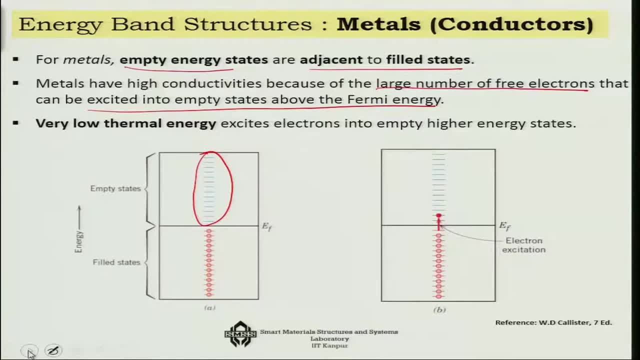 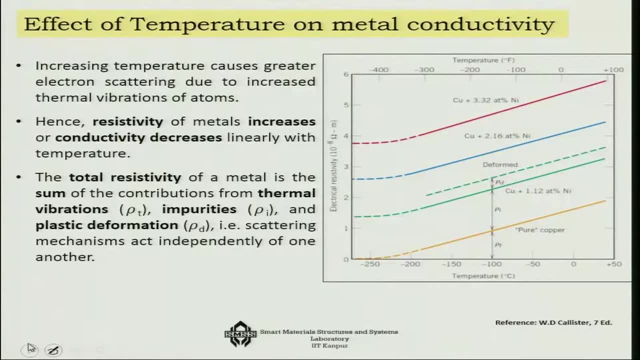 conduction, which is the, you know, conduction based on the electron flow. Now, definitely the temperature will should increase this effect. However, when you increase the temperature, it would actually cause greater electron scattering due to the increased thermal vibration of the atoms. So hence, resistivity of metals increases, or conductivity decreases linearly with the temperature. 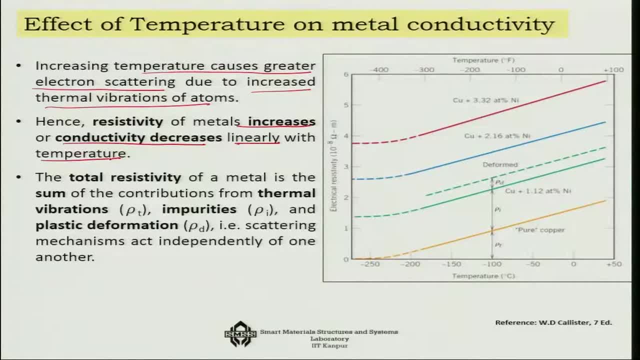 So instead of, you know, allowing the electrons to freely change this gap from the valency band to the conduction band, what happens is that it increases the electron scattering And, as a result, this free flow actually gets hampered with the increase of the temperature. 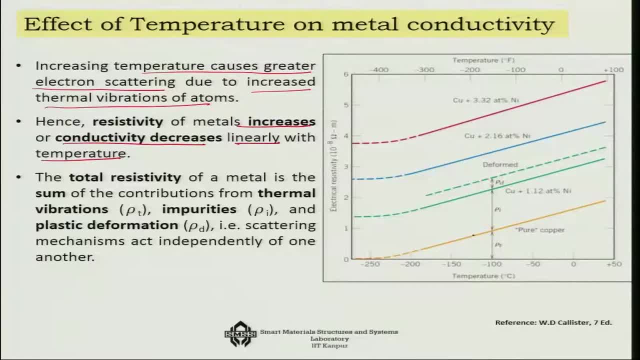 And, as you can see here in this plot, like pure copper. you know from minus 200 onwards how the resistance is. the resistivity is continuously increasing. Similarly, that is for pure copper. similarly we will see copper with nickel or you know, smaller or bigger amount. 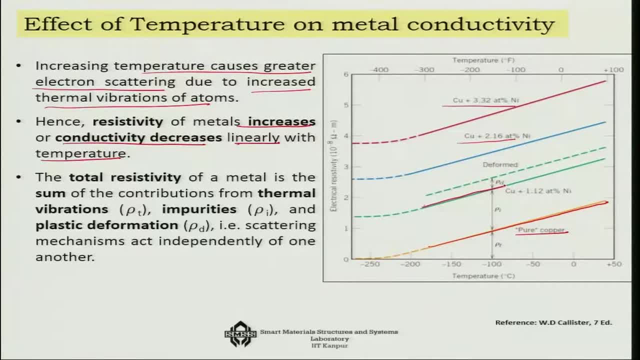 Each one of them has higher degree of resistance. Okay, It has higher degree of resistivity, but the effect is almost the similar: that it is increasing the resistivity with respect to temperature. The total resistivity of a metal, then, is the sum of the contributions from thermal vibration. 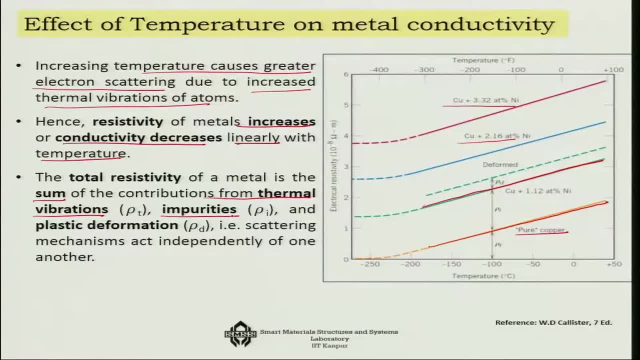 and impurities. Both of them are important, right? So, as I increase the temperature, there is a thermal vibration contribution, that is the roti, part of it, okay, And so that is the, for example, the roti, And also there are the effect of the impurities, like copper. I am adding, you know, 1.12 percent. 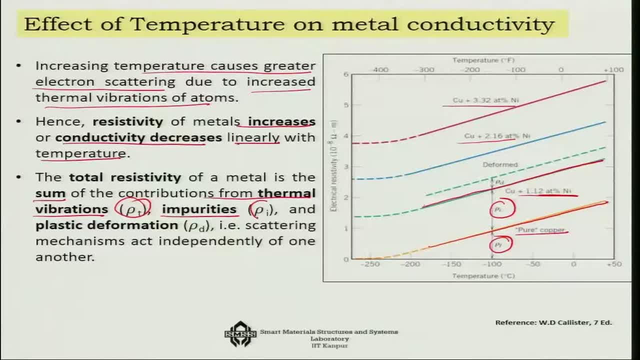 nickel. So that is the rho i part of it, the impurity part of it. Also plastic deformation, rho d sometimes. so if you further deform the same material, if you further deform it will further increase and that is the rho d. So basically total resistivity is actually part of rho d. 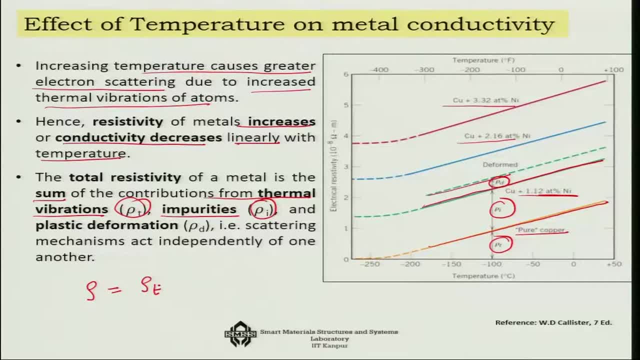 Okay, So rho t, that is the resistivity due to thermal vibration, rho i- resistivity due to, you know, the impurities. and rho d, that is resistivity due to the plastic deformation. So these are the three different things and they can act independently of one another. 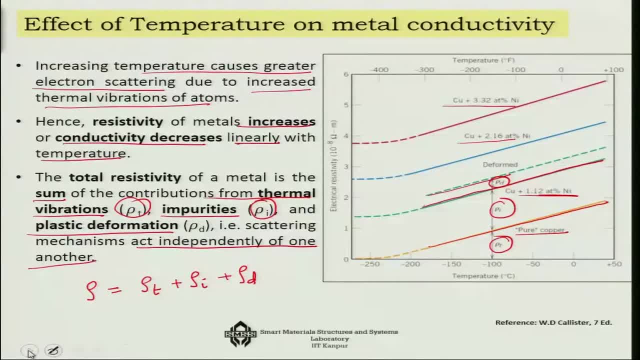 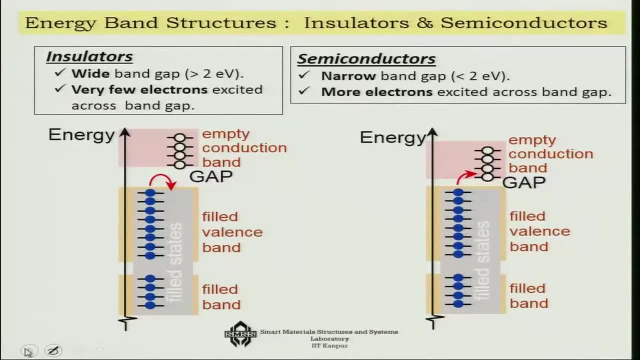 that is very important thing we have to keep in our mind. Now let us look into the energy band structures. Okay, Okay, Let us look into the energy band structure of insulators and semiconductors. Insulators: I told you that there will be, you know, a wide band gap, greater than 2 electron. 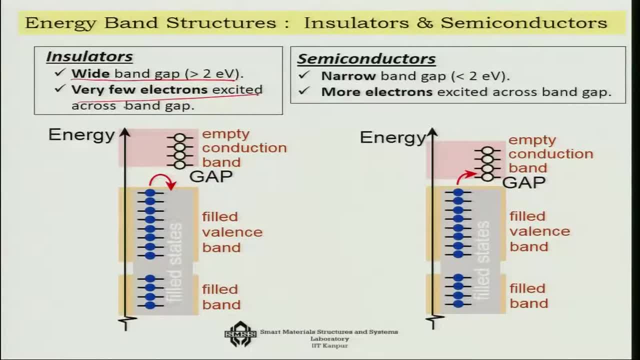 volt and very few electrons will be excited across the band gap. So you can see here that there is a wide band gap here and the conduction band remains empty. On the other hand, if you consider the semiconductor material, then there is a narrow band gap, less. 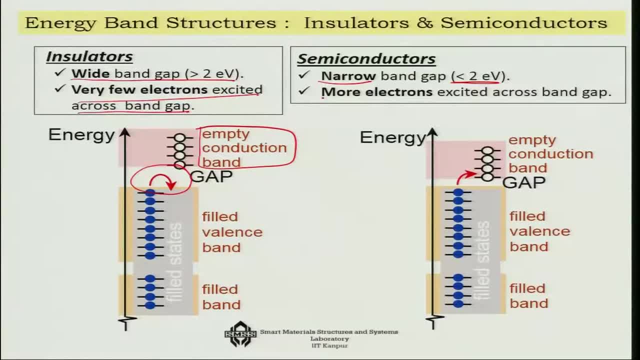 than 2 electron volt and more electrons are excited across the band gap, So more electrons can actually go from here to here. but if they go then there will be a hole formation, you know. so we will talk about it. that is the good part of the semiconductors. 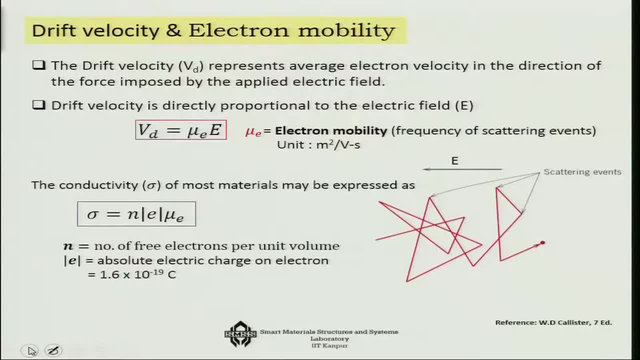 So there is a drift velocity, Vd, which represent the average electron velocity in the direction of the force imposed- Okay- By the applied electric field. Okay, So electrons, the moment you are applying the electric field, then they will start to flow and then the average velocity of these electrons is measured with the help of the drift velocity. 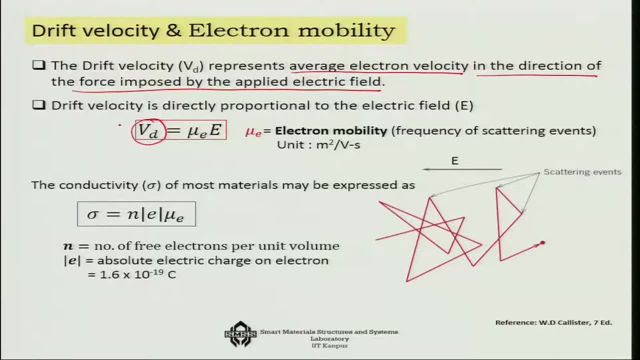 Vd, and this Vd is expressed as a function of mu 0 times the- you know- electric field E, and where mu 0 is the electron mobility, That is, the frequency of scattering, Which is measured in terms of meter square per voltage second. 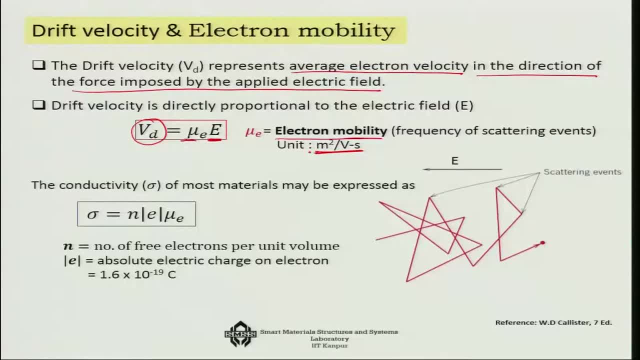 Now the conductivity sigma of most materials may be expressed in terms of this new term, mu, which is the electron mobility, and we can write it as the conductivity as N times magnitude of the absolute electric charge on electron, which is 1.6 into 10 to the power minus 9.0. 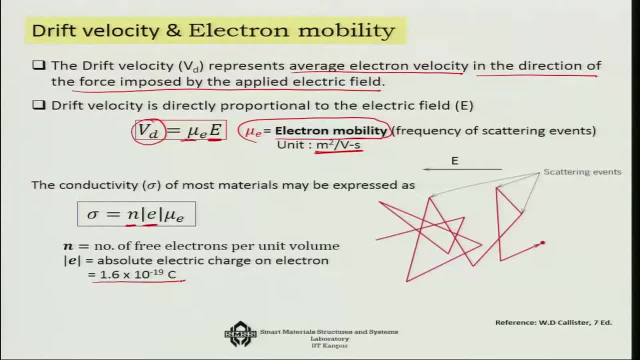 Okay, Thanks, minus 19C, multiplied by the mu E, which is the, you know, electron mobility. So if you have more free electrons per unit volume, your conductivity will be more. If you have more electron mobility, mu 0, because anyway, absolute electric charge on electron. 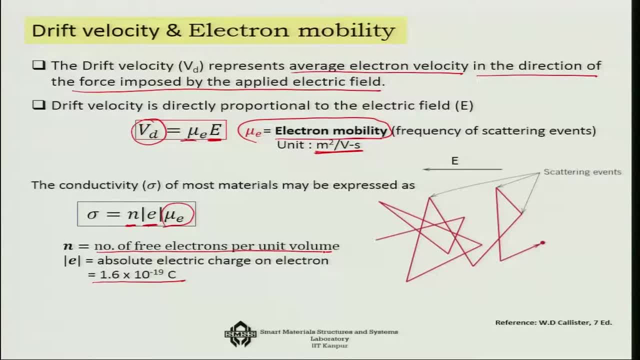 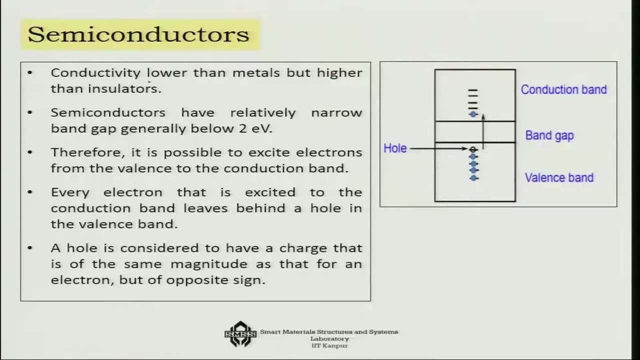 is not changing. if you have more you know electron mobility, then also you will get a higher you know conductivity in a metallic system. Now, in the case of semi-conductors, the conductivity is lower than metals, but higher than the insulators. we have seen it just now in the table. 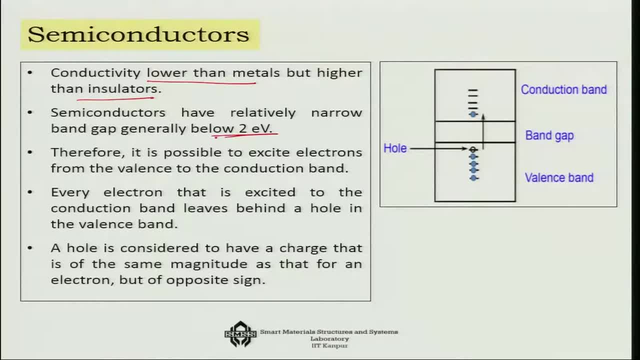 Semiconductors have relatively narrow band gap, generally below 2 electron volt. therefore it is possible to explain excite electrons from the valence band to the conduction band. Every electron that is excited to the conduction band leaves behind a hole in the valence bond, So like one electron. 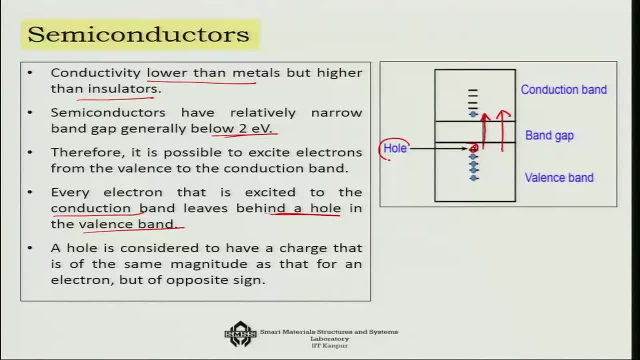 jumping from here to here. so there is a hole. there is a hole that is remaining here. A hole is considered to have a charge that is of the same magnitude as that for an electron, but of opposite sign. That is what we will call them and the electron deficiency in that. 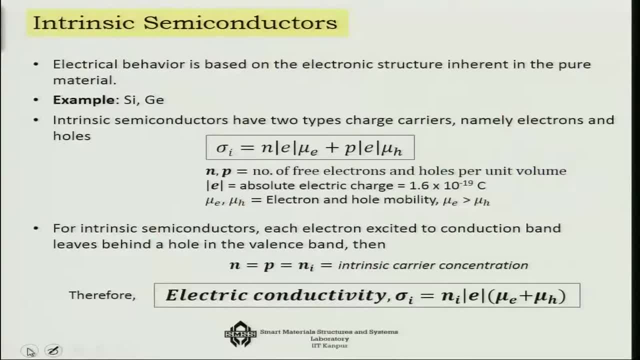 region and we will call them as a hole. Now, intrinsic semiconductors: if we consider the electrical behavior here is based on the electronic structure inherent in the pure material, For example silicon, for example germanium. Now, intrinsic semiconductors have two types of charge carriers, namely the 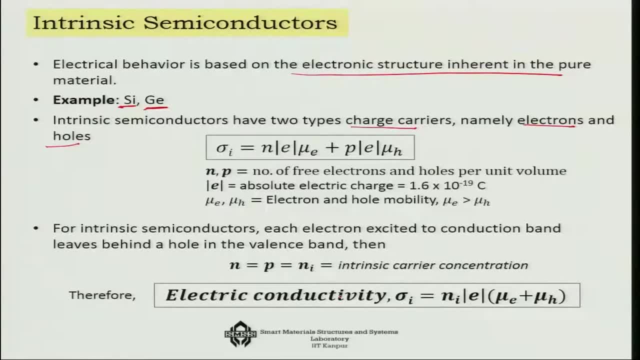 three electrons and the holes. So you can write it as n times, where n is the number of free electrons per unit volume, so n times e times mu e- electron charge mobility. and p times e times magnitude of e times mu h, where mu h is the hole: mobility. 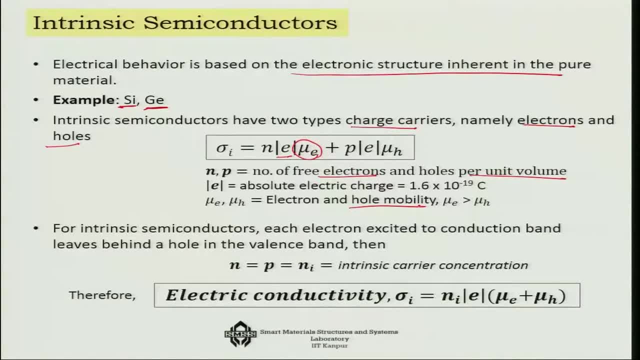 So for intrinsic semiconductors, each electron excited to conduction band actually leaves behind a hole in the valence band to the conduction band. That is why we will call themφ kind of escorto Brief Trans Attention. So you may say N equals to P, equals to Ni, that is the intrinsic carrier concentration. 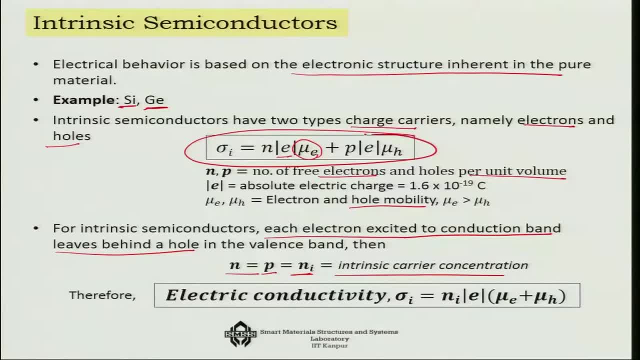 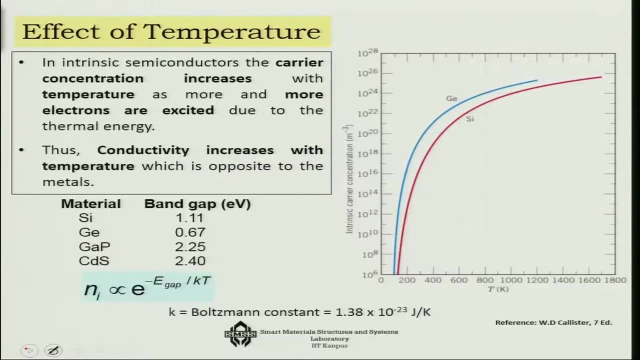 In that case you can simplify this expression further, as sigma i equals to Ni times modulus of E, times mu E plus mu H. So this is a simplified relationship of electric conductivity for the intrinsic semiconductors. What happens for the semiconductors if I increase the temperature? 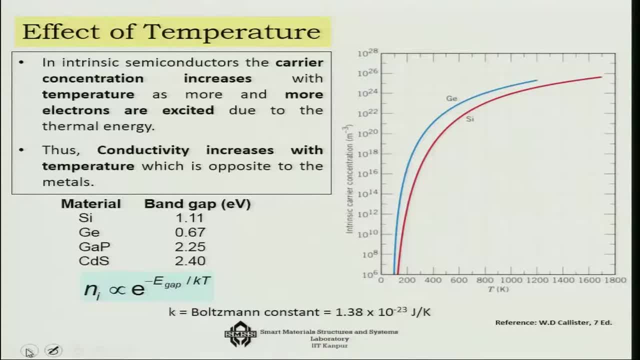 Does it behave the same way as the metals In intrinsic semiconductors? the carrier concentration increases with temperature as more and more electrons are excited due to the thermal energy and they are kind of encouraged to, you know, jump the band gap and go to the valency band. 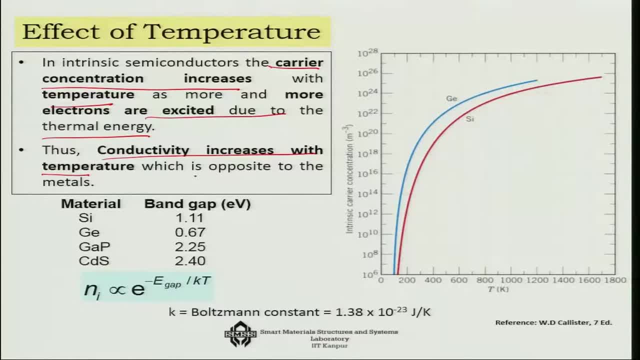 So conductivity increases here with temperature which is opposite to the thermal energy. So like silicon, the band gap is only 1.11. electron volt germanium 0.67, you know gap 2.25, cadmium sulphide 2.40. 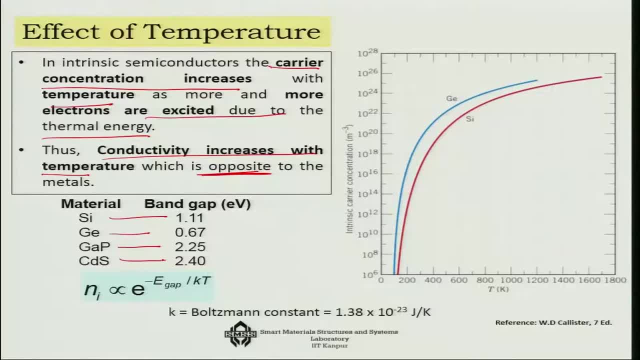 In fact you can write actually that Ni is proportional to E, to the power, you know, exponential E to the power minus E gap over kT. Okay, And k is the Boltzmann constant. So, with respect to temperature, if you plot this, you will be able to see that the intrinsic 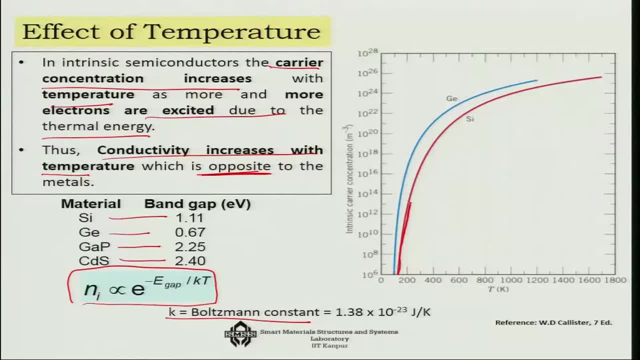 carrier concentration, how sharply it is increasing for silicon, and then it is getting saturated with respect to temperature. So similar- you know- qualitative nature you will also see for germanium. So this is opposite to the behavior that you will see in the metals. 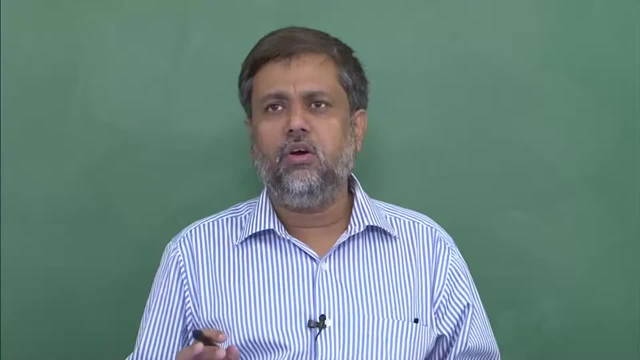 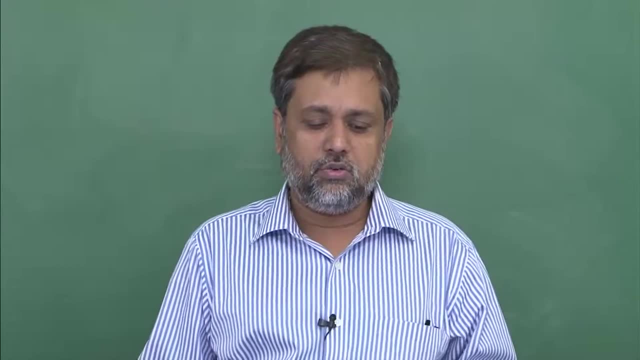 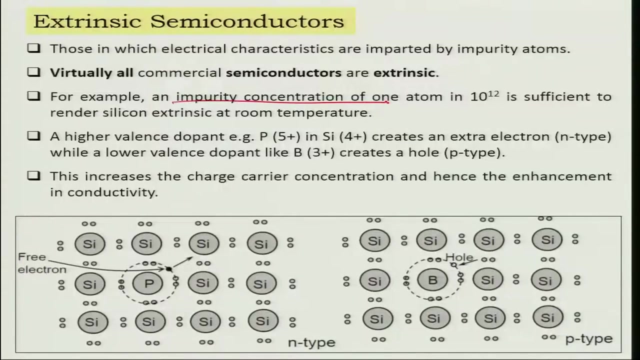 Now, very few semiconductors that we use today are intrinsic semiconductors. mostly they are extrinsic semiconductors, which means they are semiconductors because of the addition of impurity concentration, which is, you know, like something like of one atom in 10- to the 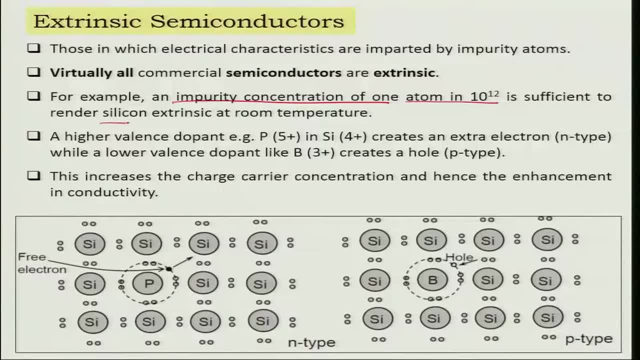 power 12 is sufficient to render silicon extrinsic at room temperature. Now a higher valency dopant Okay, For example P5 plus or silicon 4 plus. that creates an extra electron n type, while a lower valency dopant or impurity like boron or creates a hole of p type. 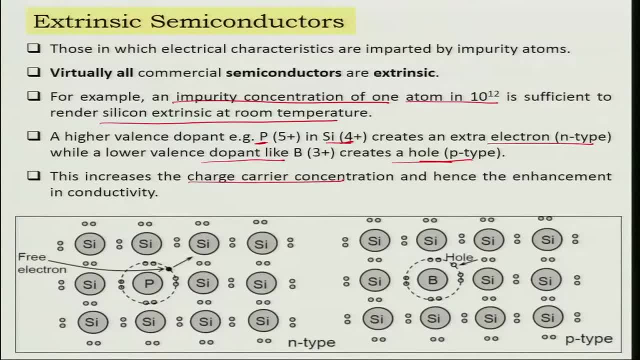 So this increases the charge carrier concentration and hence the enhancement in terms of the conductivity. So, as you can see it here that this is a silicon lattice structure and let us say you have actually added, So this is a higher valency dopant. so, as a result, this will create an extra electron. 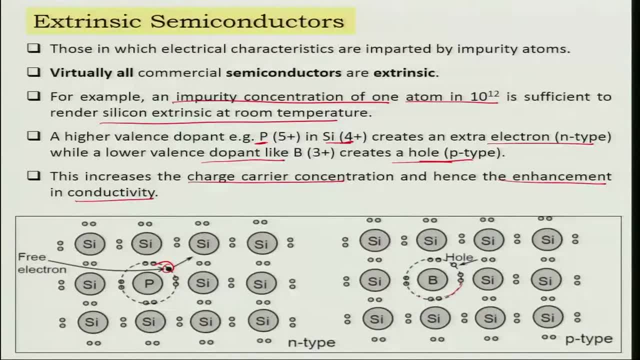 And on the other hand, if I add, you know something like boron, so this is a lower valency dopant, so electrons will travel from silicon towards the. you know this system, so thus you know one is when it is actually giving the. 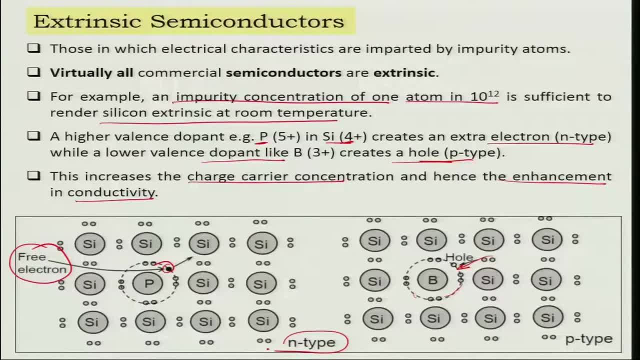 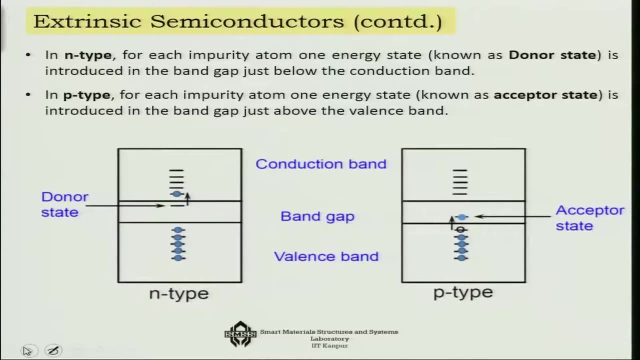 free electron, then it is n type, and when it is contributing to the making of holes, then it is actually p type. So this is the extrinsic semi conduction system. So in n type, for each impurity atom, one energy state known as the donor state is introduced. 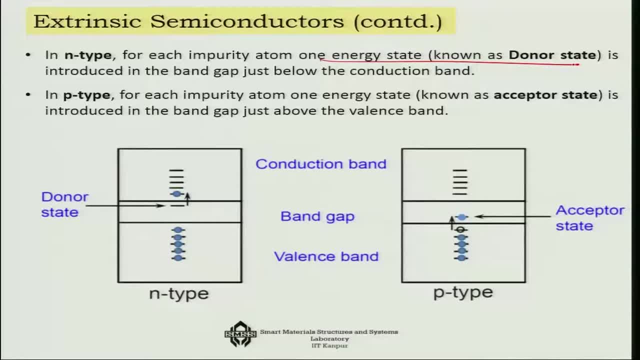 in the band gap just below the construction band, whereas on the p type, for each impurity atom, one energy state known as the acceptor state is introduced in the band gap just above the valency band, So like in the n type, if you look at it, that as the electron has travelled up. so you are. 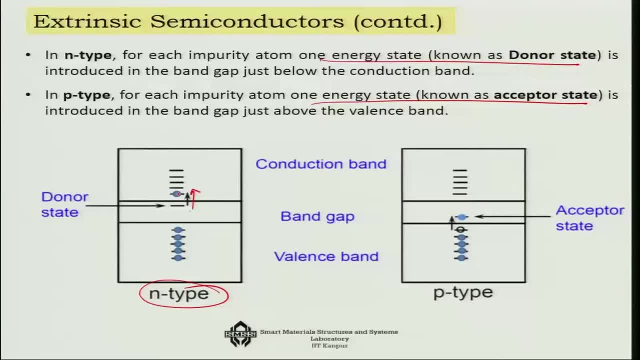 actually getting here? you know the donor state that is introduced in the band gap and on the other hand, in the p type impurity you are actually getting an acceptor state as the band gap. So this is what is the extrinsic semi conduction system. 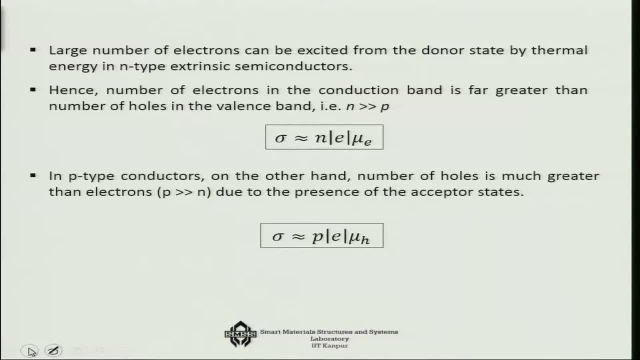 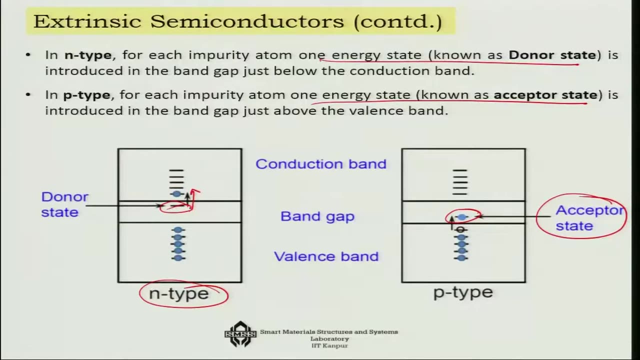 Now, large number of electrons can thus be excited from the donor state by thermal energy in n type extrinsic semiconductors. So, further to this, if you apply this, actually if we go to the last slide, that if you increase the temperature, then you can actually create large number of these donor states. 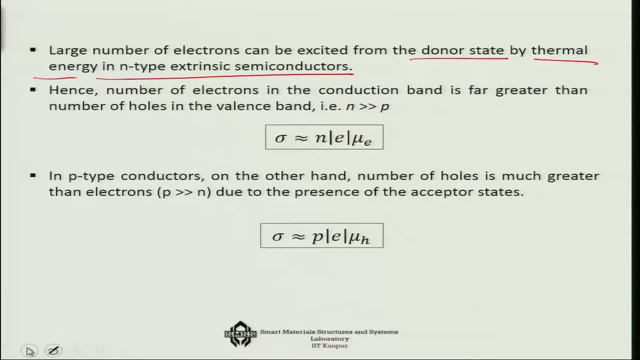 Number of electrons in the conduction band is far greater than number of holes in the valence band, and that can be written in terms of n. you know the magnitude of E times the mu E. In the case of p-type conductors, on the other hand, number of holes is much greater. 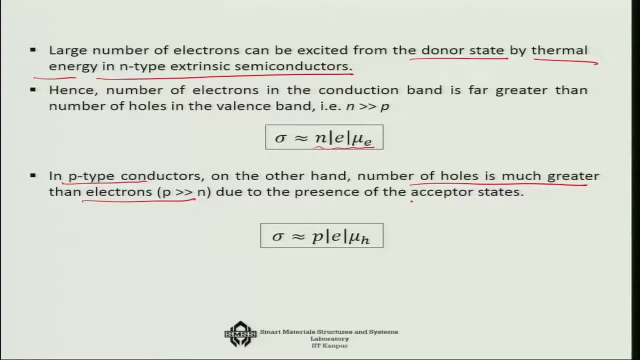 than electrons, p, much greater than n due to the presence of the acceptor states, and hence the conductivity for such material is p times, you know, p times mod of E, times mu H. So the one case it is mu E and another case it is mu H. So this point we have to keep in. 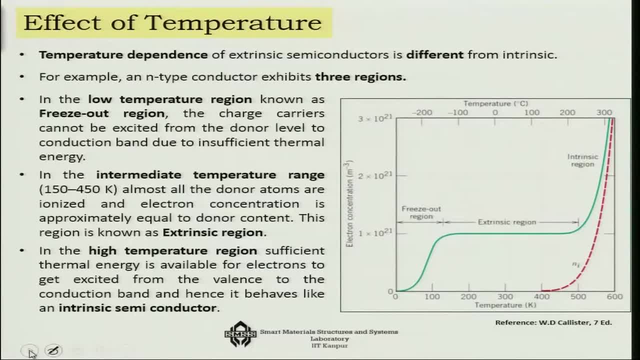 our mind Now. what is the effect of temperature in the case of extrinsic semiconductor? Here it is different from the intrinsic. For example, an n-type conductor will exhibit three ratios regions In the low temperature region known as the freeze-out region. you will see that. 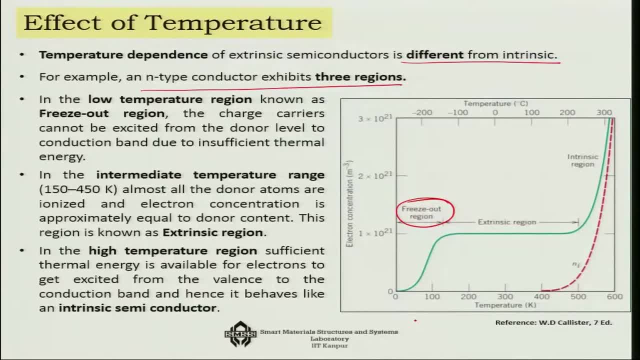 the charge carriers cannot be excited from the donor level to conduction band due to insufficient thermal energy In the intermediate temperature range. what you are going to see. so this is the intermediate temperature range. Almost all the donor atoms are ionized and electron concentration is applied. 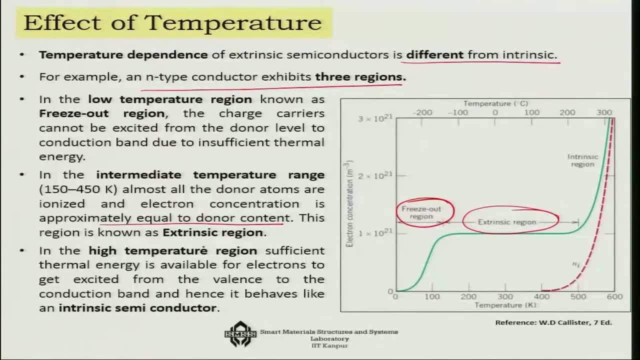 So in the intermediate temperature range the charge carriers are approximately equal to donor content. This region is also known as the extrinsic region. In the high temperature region, sufficient thermal energy is available for electrons to get excited from the valency to the conduction band, and hence it behaves like a intrinsic semiconductor. So, with respect, 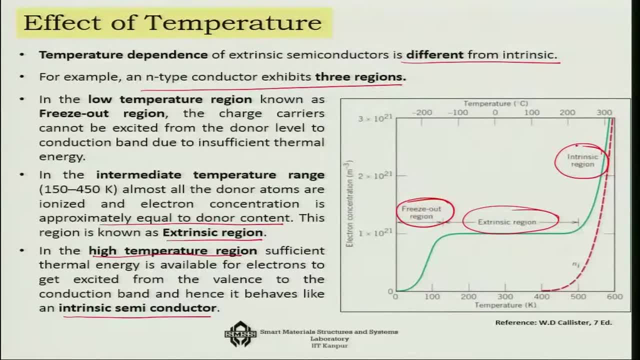 to temperature, you have these three regions: the freeze-out region, extrinsic region and intrinsic region. In the extrinsic region, the temperature is high In the intermediate temperature range region, as you can see that the electron concentration is remaining almost constant. and then, as you, 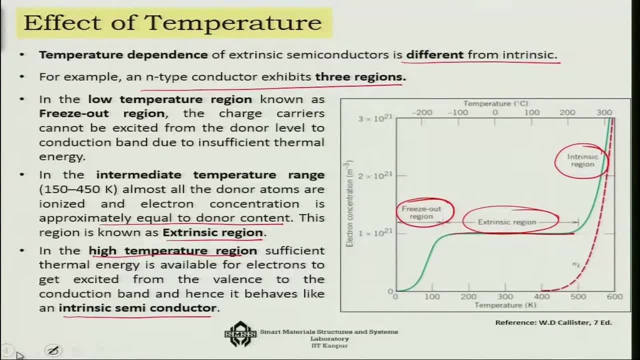 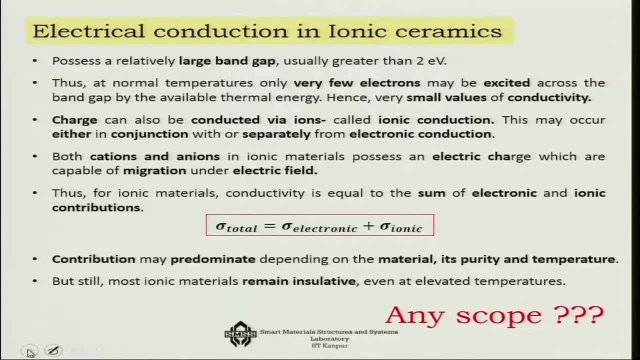 are increasing temperature, intrinsic region is getting dominant in the system. Now you know, in terms of the ionic ceramics it possess a large band gap. usually it is greater than 2 electron volts, like the semiconductor materials, Whereas at normal temperature only very few electrons may be excited across the band gap. 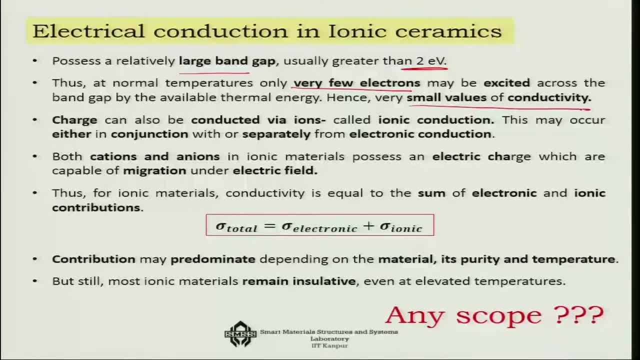 by the available thermal energy. hence it has a very small value of conductivity. However, for the ceramics, I told you this point earlier that it can also be conducted by ions called ionic conduction. This may occur either in conjunction with or separately from electronic conduction. 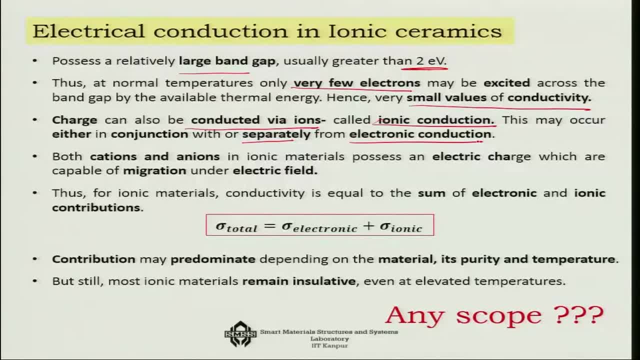 So there is a new thing that you have, which is the ionic conduction. Both cations and anions in ionic materials possess an electric charge, which are capable of migration under the electric field. Thus for ionic materials, conductivity is equal to the sum of electronic and ionic contribution. 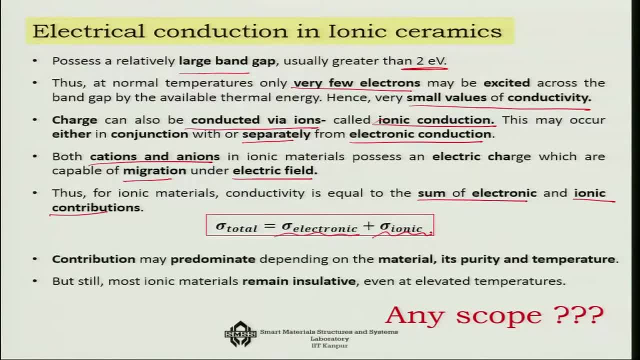 So their conductivity has electronic contribution and an ionic contribution. Now this contribution may predominate depending on the material, its purity and temperature, But still most ionic materials remain, you know, insulative, even at elevated temperatures. So can you think of any scope of applying this particular property? 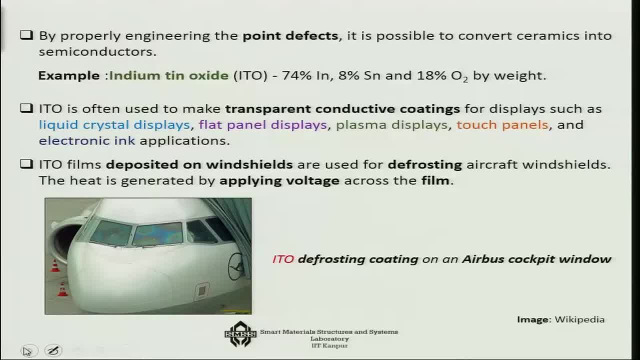 For example, we can tell you that one such interesting thing- that by properly engineering the point defects, it is possible to convert ceramics into semiconductors. Example: if you make indium tin oxide, ITO- This is the point defect- It has 74% indium, 8% stannium and 18% oxygen bioate. 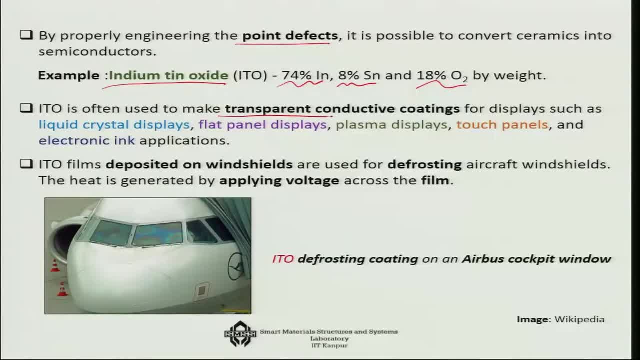 ITO is often used to make transparent conductive coatings for displays such as your LCD display, flat panel display, plasma touch panels and electronic ink applications. In fact, if you look at the aircraft, then on that window you use ITO films deposited on. 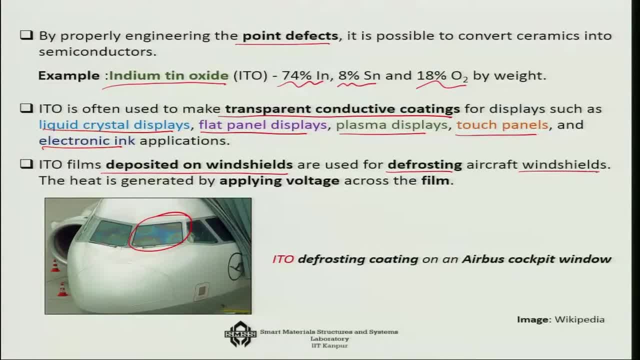 windshields, which are used for defrosting aircraft windshields, The heat is generated by applying voltage across the film. So thus you know, by properly engineering point defects, you can actually convert the ceramics, at least, to the semiconductor level. And ITO defrosting coating on an air bus cocktip window is what you know. is can be taken as: 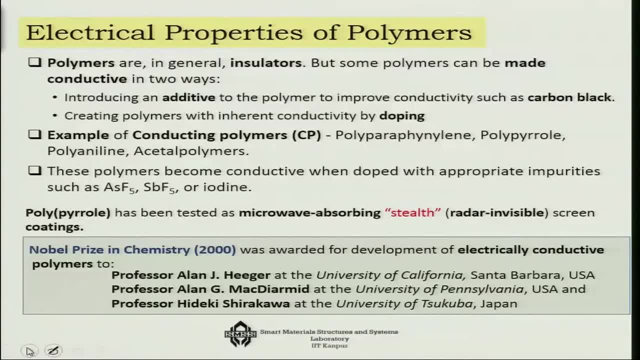 an example of the whole thing Now, in terms of the polymers. Polymers are, in general, insulators. They are much more insulators than the ceramics. But some polymers can be made conductive in two ways. One is introducing an additive to the polymer to improve conductivity, such as carbon black. 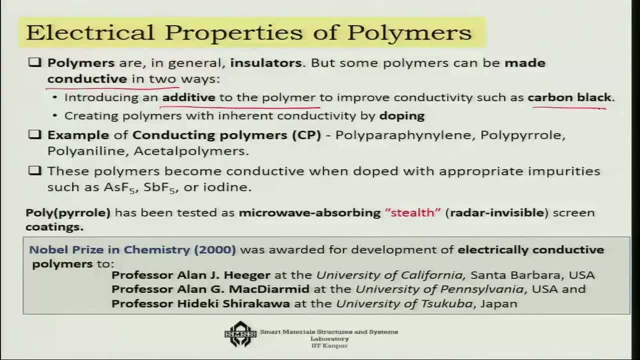 graphite pellets or even silver, you know flakes you can use. The other is creating polymers with inherent conductivity by doping. Example of conducting polymers are like this: Polymers are like polyparaphynylene, polypherol, polyaniline acetyl polymers. 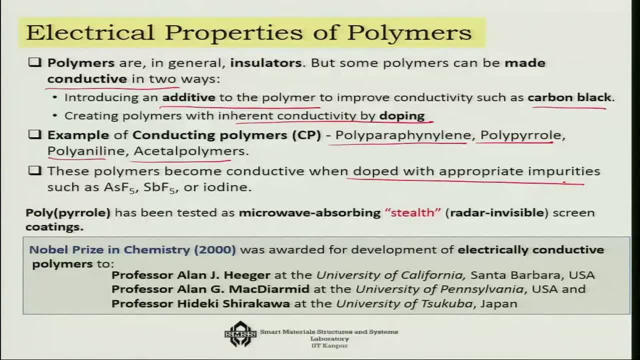 So these polymers become conductive when doped with appropriate impurities, such as ASF5, SPF5 or iodine Polypherol has been tested as microwave absorbing, so stealth, you know, rather invisible screen coatings. It is interesting to note that in 2000 the Nobel Prize was awarded for the development.